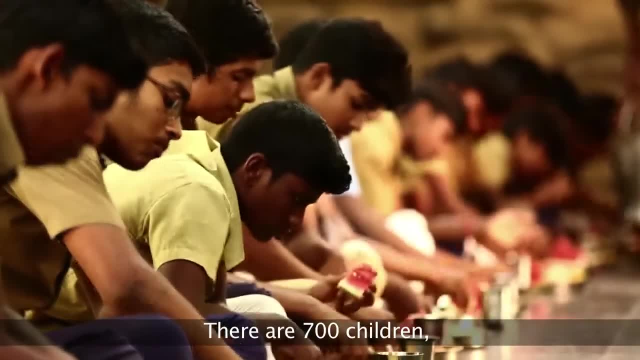 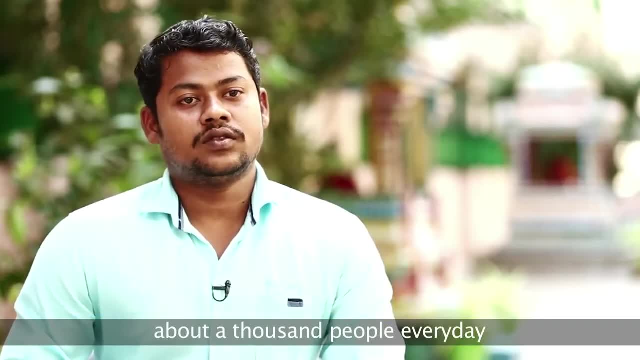 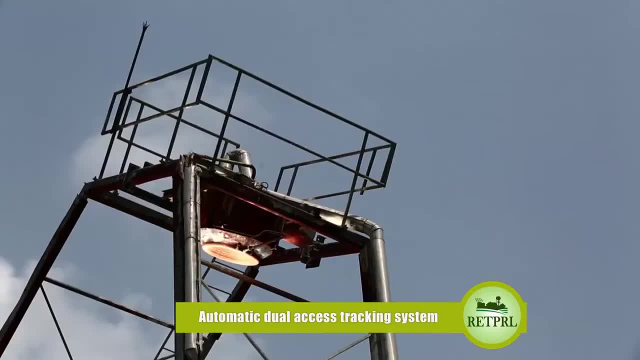 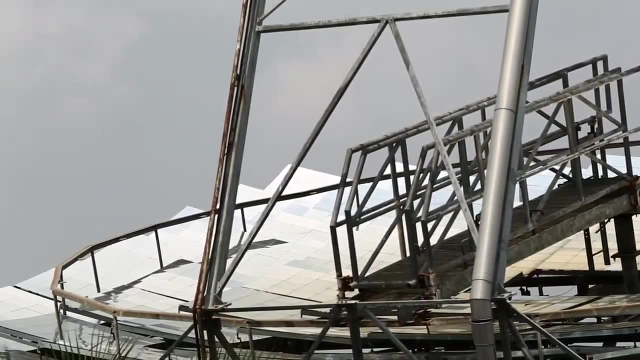 There is a lot of work to be done. There is a lot of work to be done. The Arun Thermal Dish has an automatic dual access tracking system. Once installed, it always focuses the sun. The dish concentrates the solar energy falling on it towards the solar boiler fixed on the top centre of it. This increases its temperature. 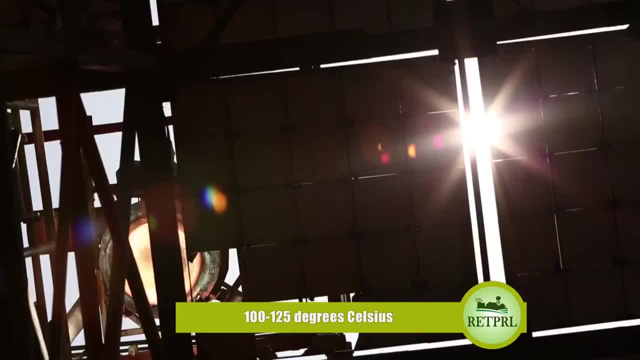 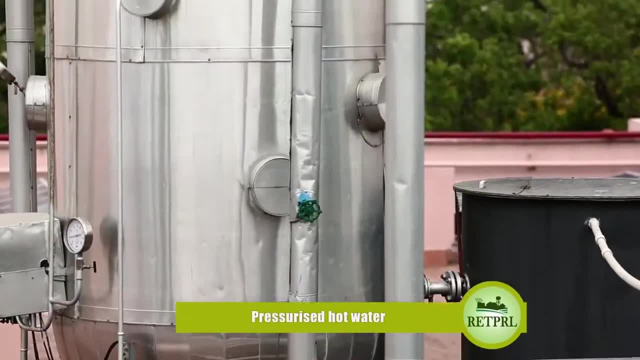 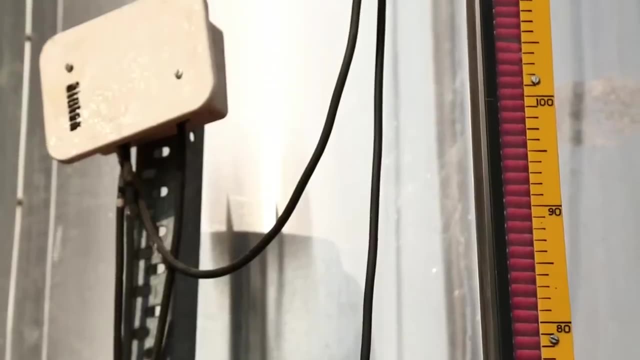 up to 100 to 125 degrees Celsius. Water supply is connected to the boiler through pipes. Hence steam is produced, is generated, which goes to the accumulator where it is stored as pressurized hot water. the temperature thus increases with pressure up to 125. 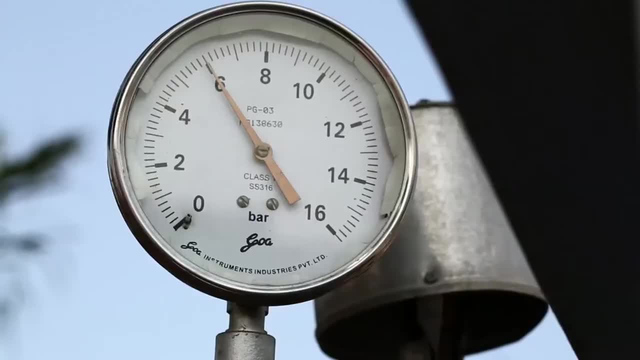 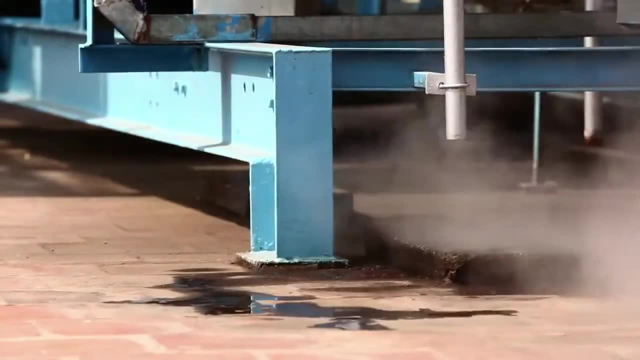 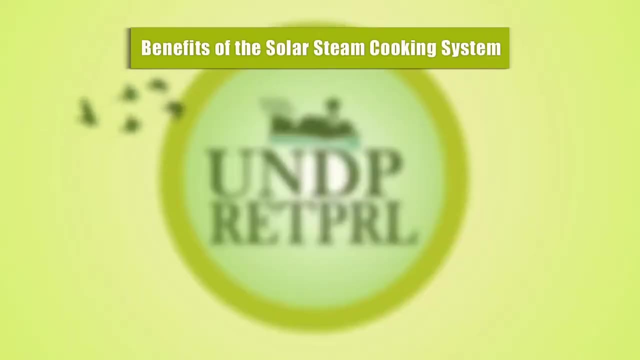 to 180 degrees Celsius. the pressure handled is from 1 bar to 8 bars, but cooking requires only 1 bar. hence the excess pressure is released through a valve and the steam sent to the kitchen through pipelines. benefits of the solar steam cooking system: LPG usage reduction of 25 to 30 percent, 35 to 40. 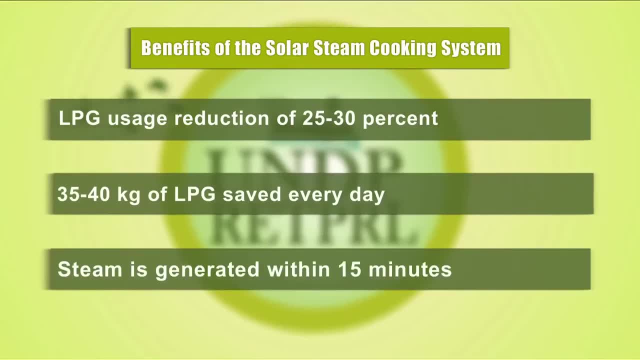 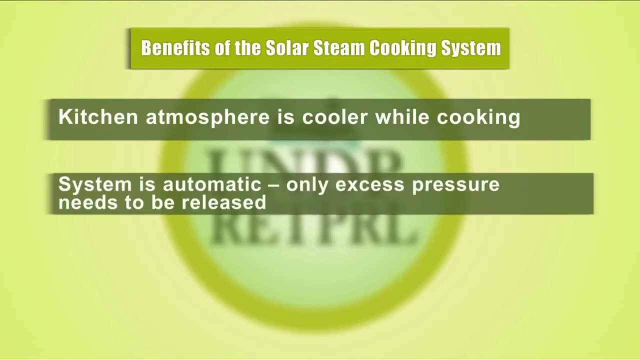 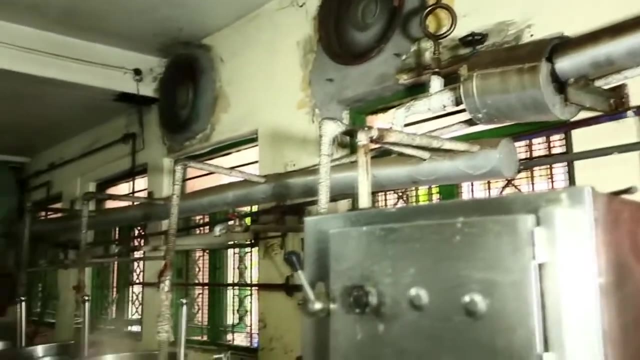 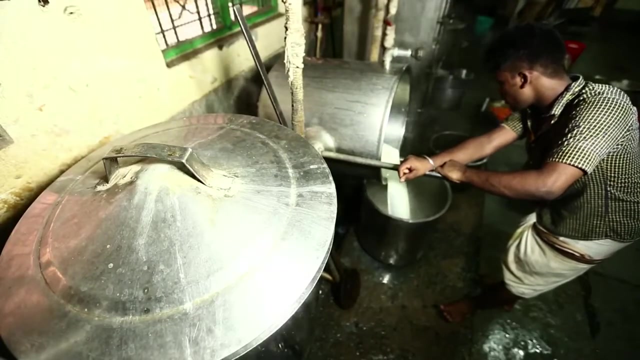 kilograms of LPG saved every day. steam is generated within 15 minutes, kitchen atmosphere is cooler, while cooking system is automatic. only excess pressure needs to be released. the solar steam cooking system is used to make vegetable dal, rice, idlis, etc. it is also used to boil milk. however, for seasoning and frying, LPG has to be. 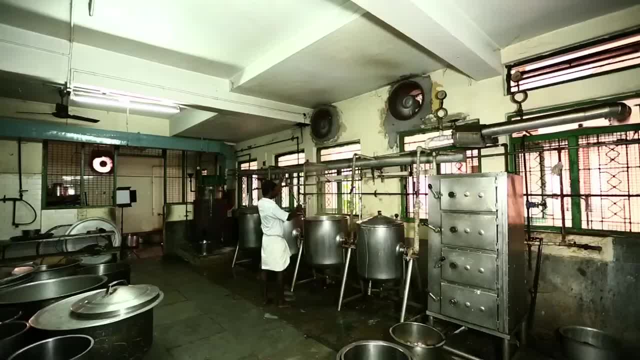 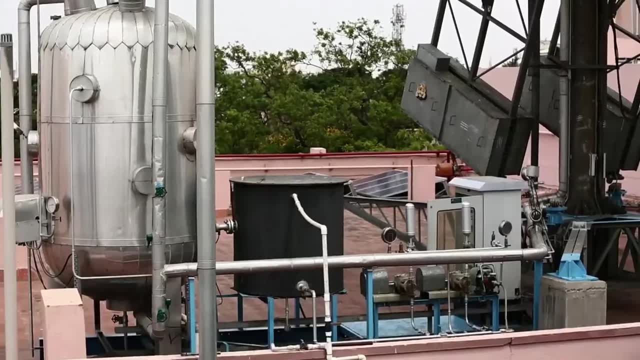 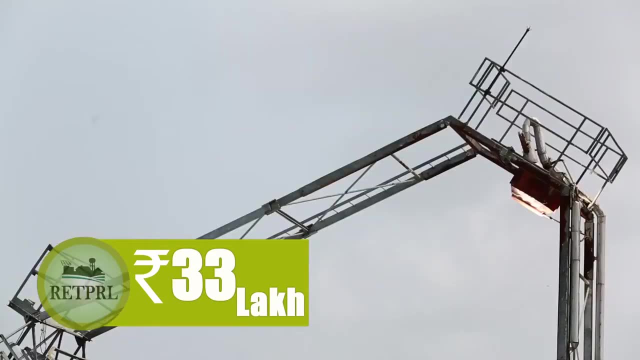 used four to five men cook the food. the kitchen is cooler as the inside atmosphere is not heated up directly, unlike in the case of LPG. because of the stored steam, the system works even during cloudy weather. this solar thermal based system costs 33 lakh rupees. 30% of the amount was provided by MNRE and UNDP.